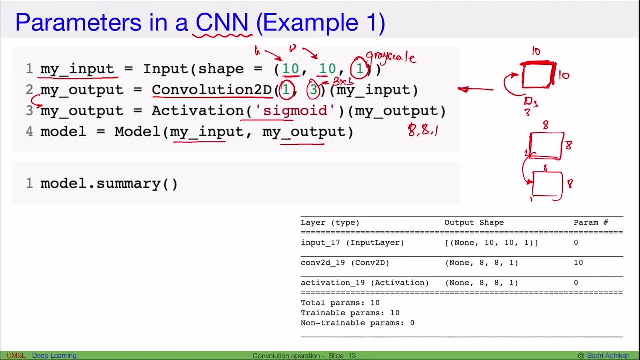 And this becomes my input, becomes my input and my output becomes my output. So if we summarize, if we run modelsummary for this model, then we see that our input, our first layer, input layer, is 10 by 10 by 1.. 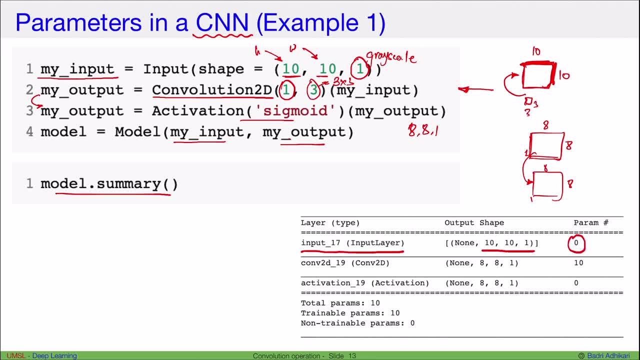 It has zero parameters because we are using input as it is, Our conf 2D layers. output is an 8 by 8 by 1 output And the total number of parameters it has is 10.. So how does it have 10 parameters? 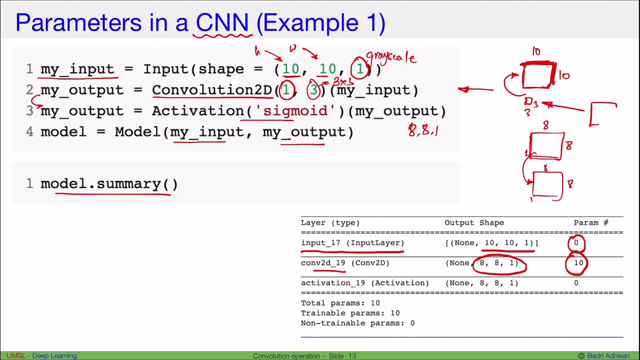 It has 10 parameters because this is a 3 by 3 filter, So obviously there are 9 values plus every filter has a bias associated with it. So 9 filter values plus 1 bias gives us 10 parameters for the filter. 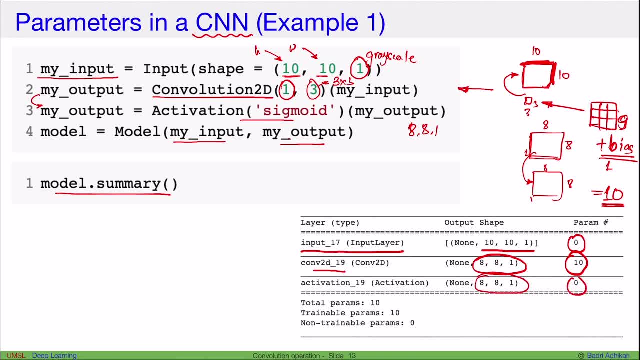 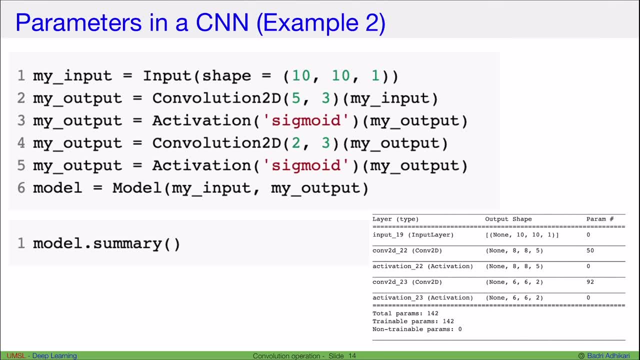 And the activation is still produced, It maintains the shape, it has zero parameters. so we get total 10 parameters for this convolutional neural network. Let us look at another example. So in this case we have once again image of size 10 by 10 by 1, only one channel as input. 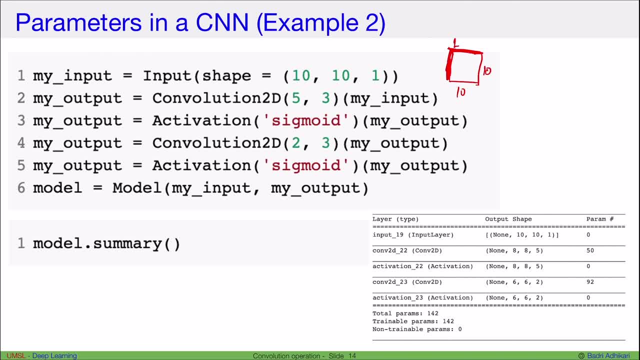 So this is again a grayscale image: 10 by 10 by 1.. In the next layer we have a convolutional layer with 5 filters, each of size 3 by 3. So we have 3 by 3 filter, another 3 by 3, another 3 by 3.. 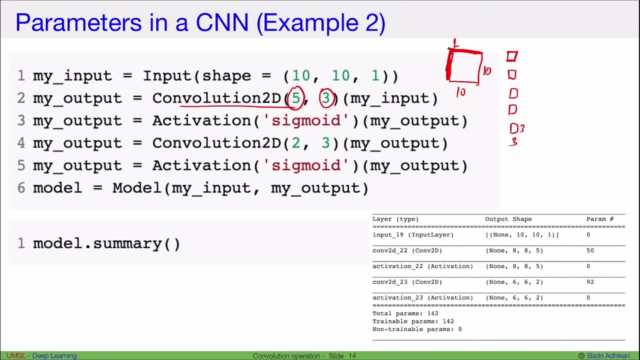 We have total 5, 3 by 3 filters: Filter number 1,, 2,, 3,, 4, and 5.. So when we apply these 5 filters into my input feature map, the output I am going to get is the first one gives me 8 by 8 by 1 input. 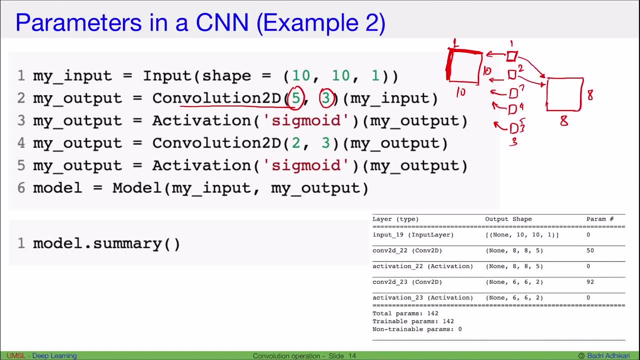 This is from the first filter. The second Filter will give me something similar, but as a different channel. The third filter gives me one more channel. Fourth and fifth give me two additional channels, So my output is actually 8 by 8 by 5.. 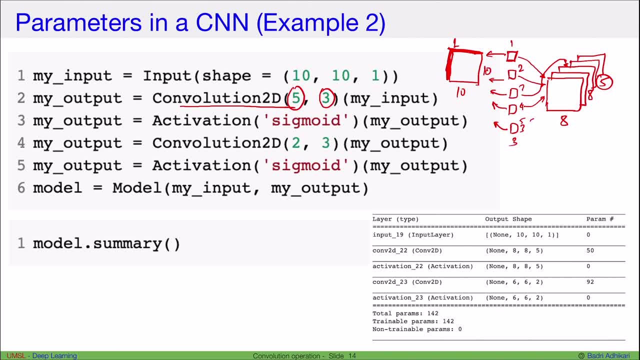 I have 5 depth here. So, as we can see, the input is 10 by 10 by 1.. The next filter, the next layer, we have 5 filters. This gives me an output of 8 by 8 by 5.. 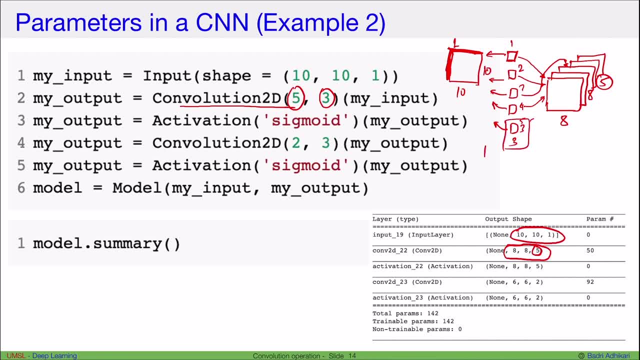 The total parameters That we have is: each filter has 10 parameters associated with it. Since I have 5 filters, it's 5 times 10, 50 parameters. The next is sigmoid layer. So all of these go through sigmoid, but the shape stays the same. 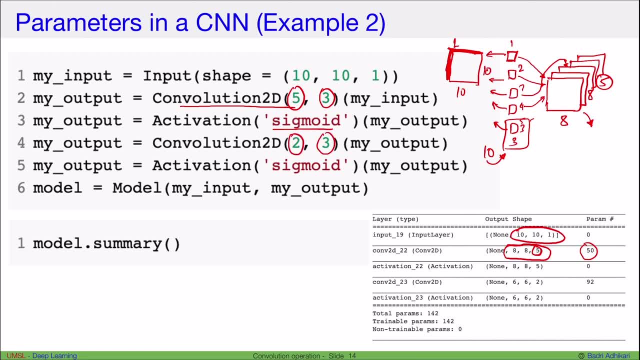 In the next layer I have two convolutional filters, each of size 3 by 3.. So if I apply two convolutional filter, each of size 3 by 3. So I have 3 by 3 filter, once again 3 by 3 filter. 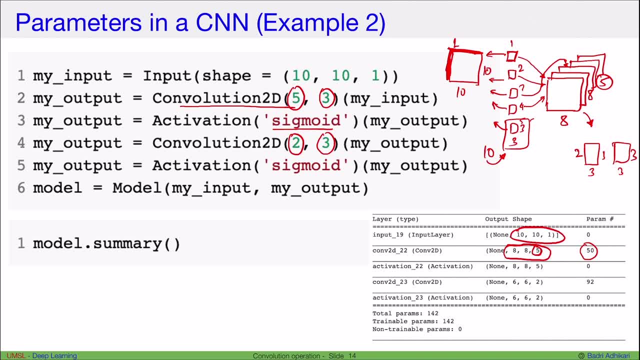 Now 3 by 3 filter. This is where things get tricky, So let me focus only on the first filter. So let me erase this and let me focus on the first filter of size: 3 by 3.. Now for this filter to convolve through my input volume, which is 8 by 8 by 5,. 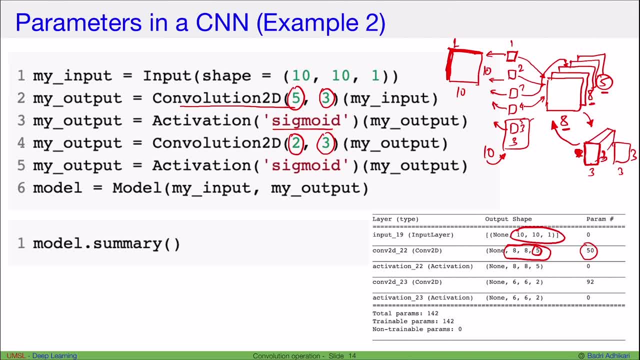 this filter must be of depth 5.2. So this filter should actually become a volume of size 3 by 3 by 5.. In order for me to convolve, I have to convolve through one piece of this input. So now we have. so when we when I convolve a 3 by 3 by 5 filter on this 8 by 8 by 5 filter. 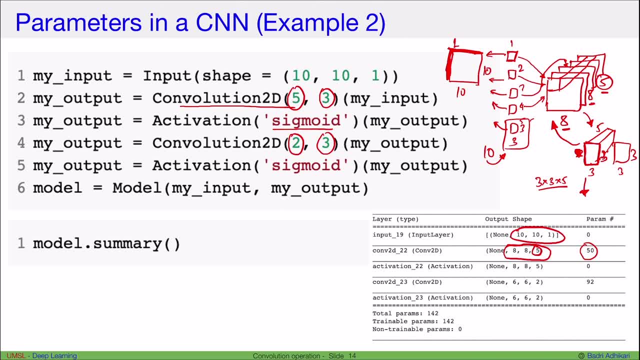 the output that I'm going to get is 8 minus 2, 6 by 6 by 1 output, And since I have two filters like these, the output will be 6 by 6 by 1.. So these two concat. 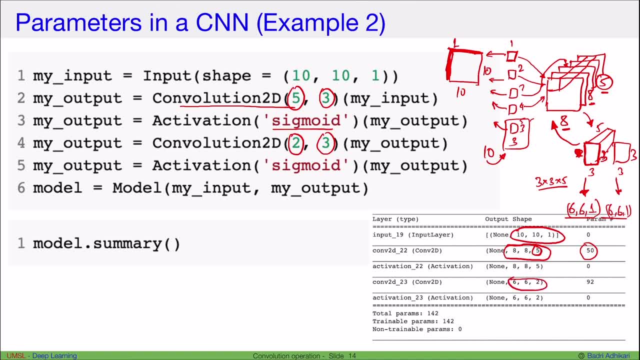 then makes it 6 by 6 by 2. And the total number of parameters is one filter has 3 by 3 by 5.. This is 15 times 5, is 45 parameters plus one bias. That makes it 46 parameters. 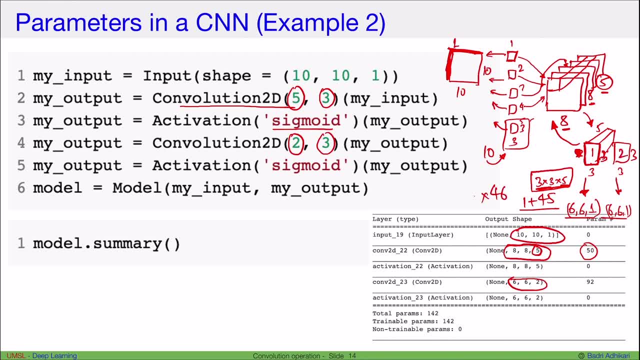 And since we have two filters, filter one and filter two, this is 46 times two, gives me 92 total weights parameters. And then we have sigmoid at the end, So this is 2.5.. So this output of size 6 by 6 by 2 gets passed through the sigmoid. 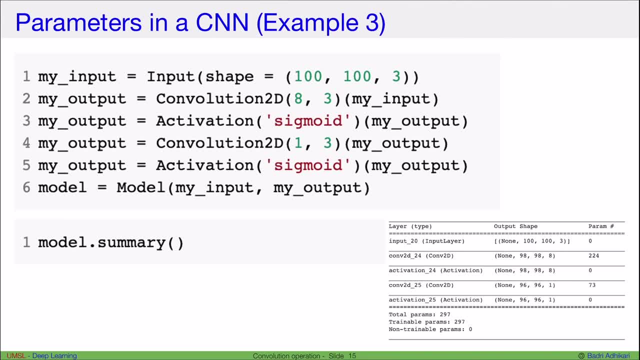 And then the output remains at 6 by 6 by 2.. Here's another example. So the input here is a 100 by 100 by 3 image. So this is a color image. My input image is 100 by 100 by 3 because I have three channels. 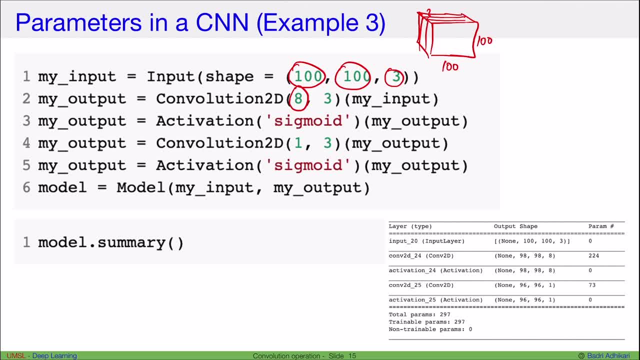 And in the first phase I'm applying 8, 3 by 3.. Convolutional filters So 1,, 2, 3, 4, 6, 7, 8, each of size 3 by 3.. 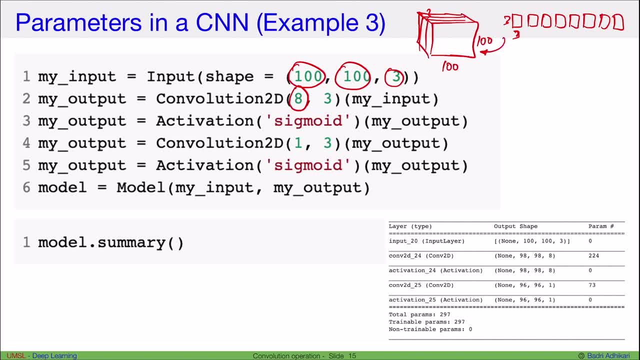 So once I apply convolution 3 by 3 through this, the output I'm going to get is 98 by 98, by the number of channels I'm going to get is equal to the number of filters. This is 8.. So the output becomes 98 by 98 by 8, which you can see that the output column has 98 by 98 by 8.. 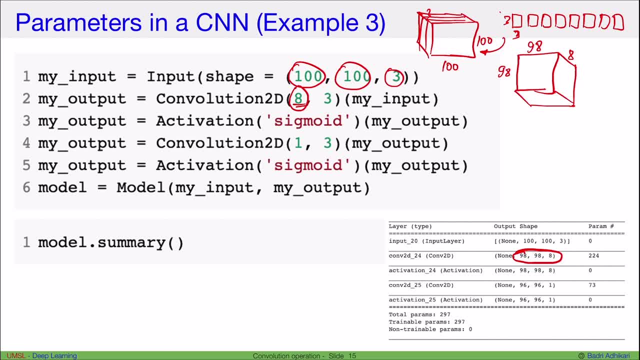 And the total number of weights we have is: each neuron has 10 parameters associated with it. Well, actually not 10.. Here's why it's not 10.. It's not 10 because, in order for the filter, so each of this one filter that we have, in order for this to multiply with my input, portion or crop of my input, correctly, 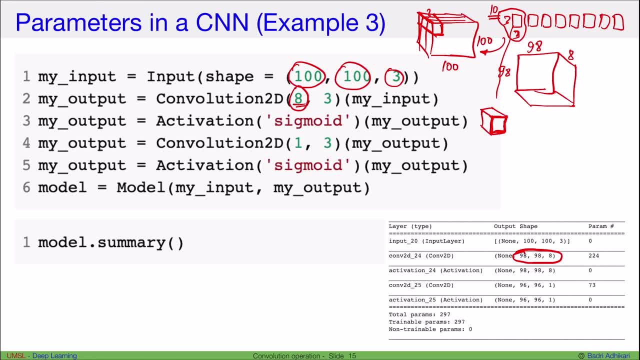 this filter must be of the same depth, So it should be 3 by 3 by 3.. So the filters automatically adapt to match the number of channels in the input. So here now, the filter number of weights in this filter is 27 plus one bias makes it 28.. 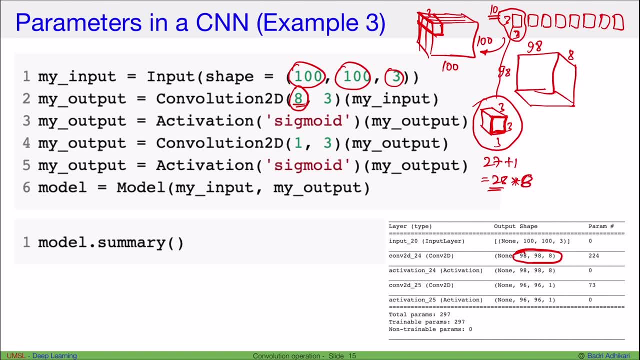 So 28 times 8, because we have 8 filters- gives me 224.. Here's the 224 number of parameters we have. So the output that we get now is a 98 by 98 by 8.. eight volume. then we apply sigmoid. this doesn't change anything, and then we apply: 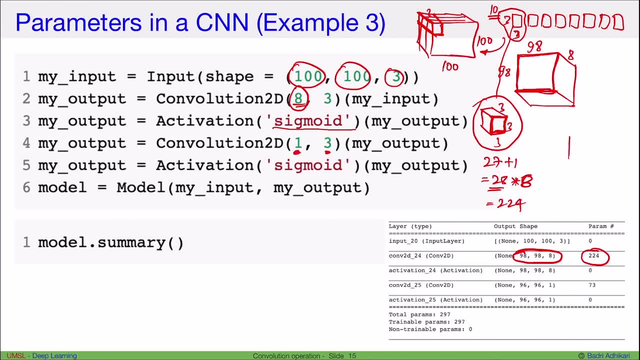 a one convolution of three by three filters. so i have a three by three filter. now it has to match the input depth, so this, the number of depth in this filter, is also eight. so i have three, three, nine, um, and nine times eight is um, 72 number of weights here in my filter. so this convolves: 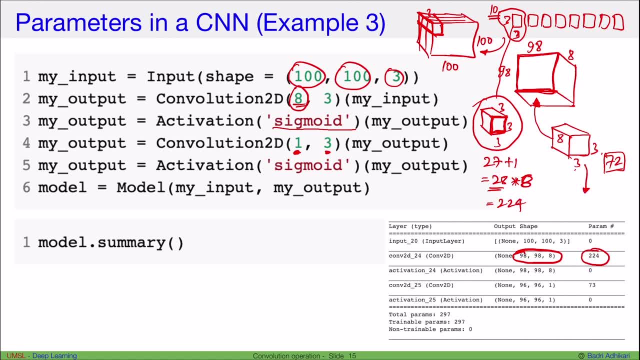 through my input volume and what comes out is a single value. um sorry, actually, what comes out is: so this is a three by three united. when i did so, what comes out is 96 by 96 by one, because we only have one filter. so this gives me output volume, but only one channel of 96 by 96 by one. 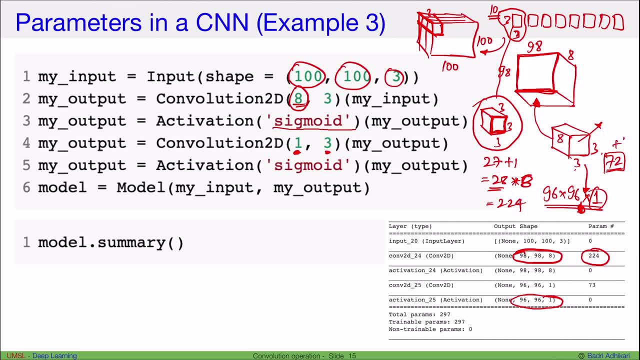 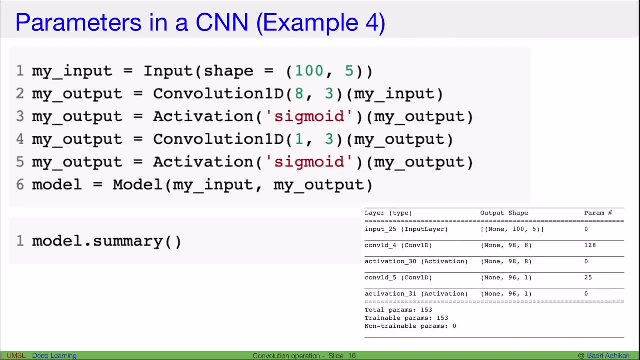 and the number of parameters here are 72 plus one bias gives me 73 weight parameters here associated with this filter. here's another example of a convolutional network, and this one is a little different because here we are looking at 1d convolutions, just the. 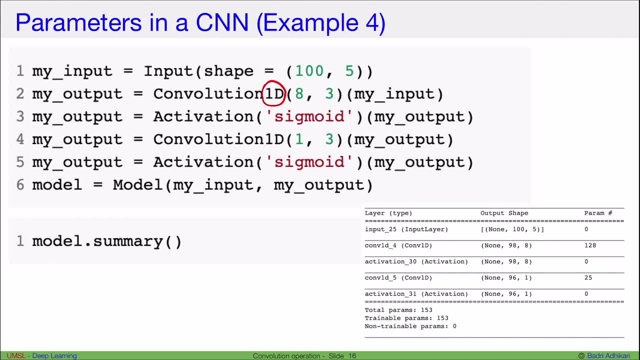 way we can do 2d convolutions, we can also do one dimensional convolutions, and here the input is of length 100 and has five channels in it. so the input is 100 length and the number of channels is five. so it has actually has. 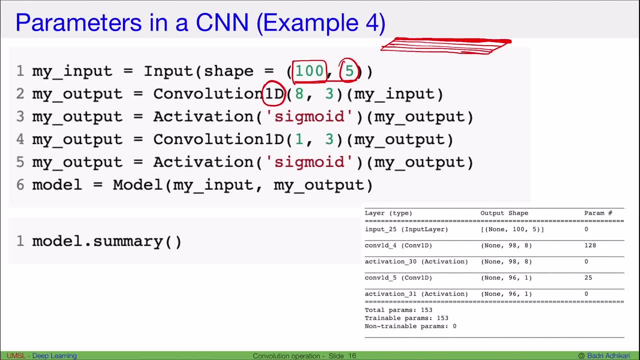 five sort of rows of data in it. in the first round i apply eight filters, each of size three. so each of size three means i'm going to look at three values at a time, and there are eight of them, so if i had. so what we have is one, two, three. so this is my first filter. 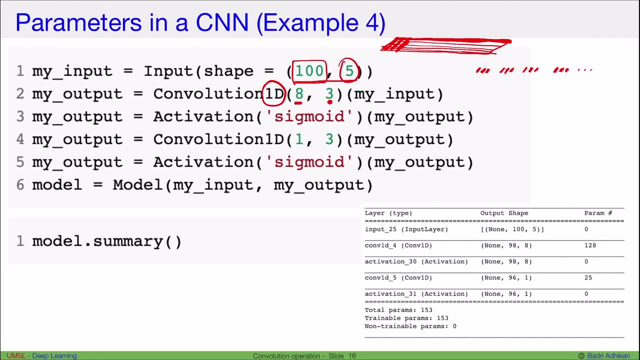 second filter, third filter, fourth filter and so on. i have eight of them. so when we convolve the first input, 100 by five, with my first filter, of course it has to. it's a three by three filter. it has to match the input number of channels, so this becomes not just three filter but three by 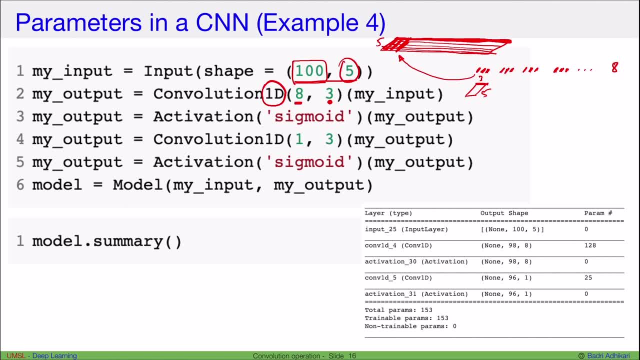 five filters so that it matches. this is five, it matches the input. so then, what comes out of this? since this is a three by three filter and the length is hundred, is actually a 98 length vector- 98 length vector. well, after we apply this filter, convolve through this filter, now we have eight of 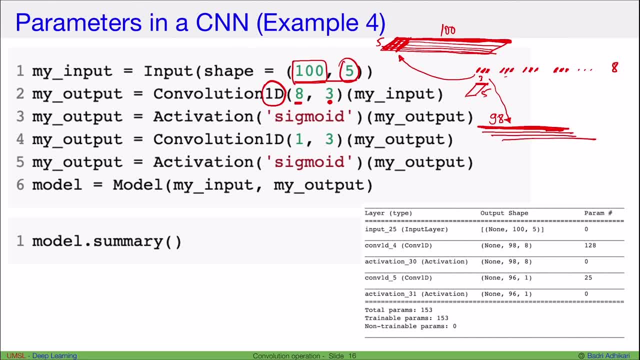 these. so we have 98 by 8 as our output, 98 by 8 as our output. the number of weights associated are: each filter has these 5 times 3, 15 parameters, and 15 plus 1 bias is 16 parameters. so we have. 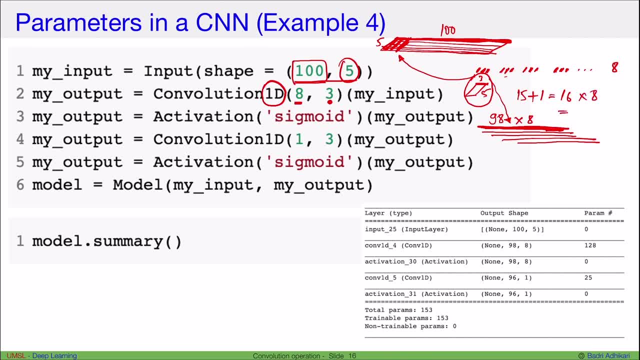 8 filters total. so 16 times 8 gives me 128.. so this is the number of parameters we have, and the output of convolving is 98 by 8.. so then we apply sigmoid, doesn't, doesn't change the dimension. so now for this 98 by 8 input. then